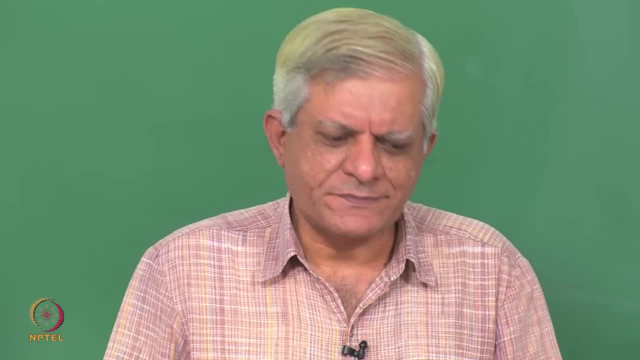 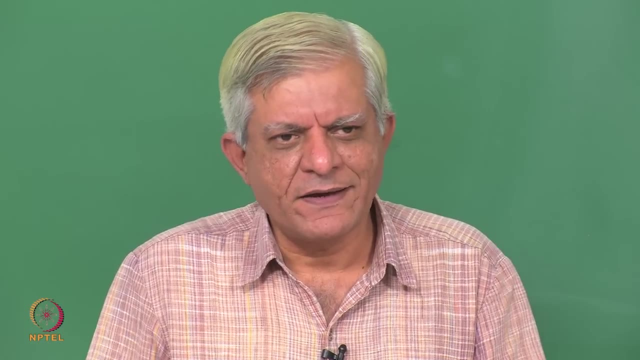 we have the context amongst everybody that what is the meaning of what we have written essentially Now? in this context, I may say that when you often write programs, you use words which are meaningful to you. So instead of writing i and j, you might use a word like count or 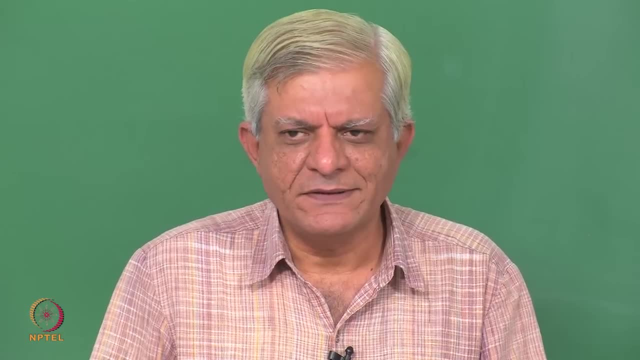 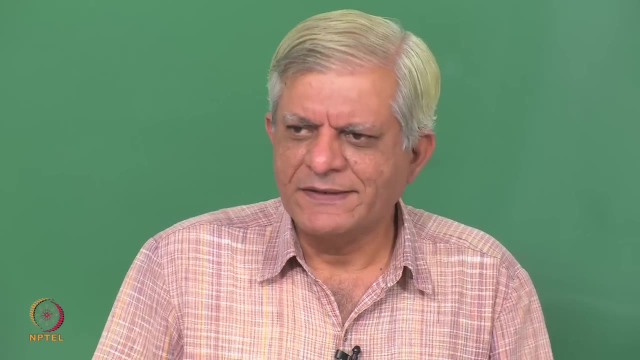 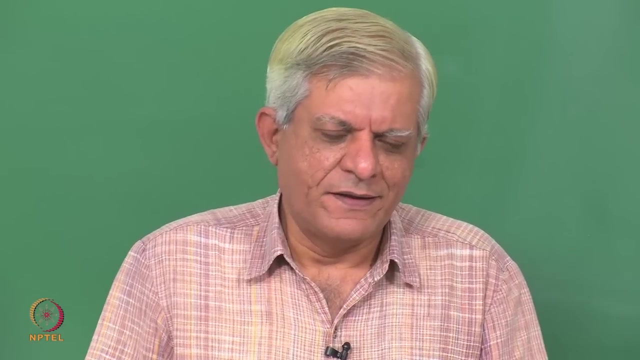 total marks or marks and things like that for variables, and you may store some numbers in that. Now when we talk about semantics we do not really look at the English we are meaning of that word. So if I write, count is equal to count plus 1, it is only for my. 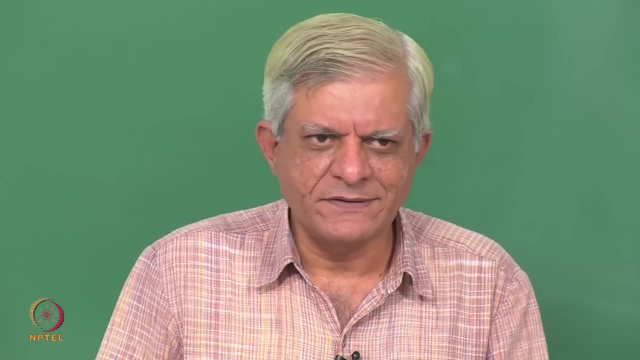 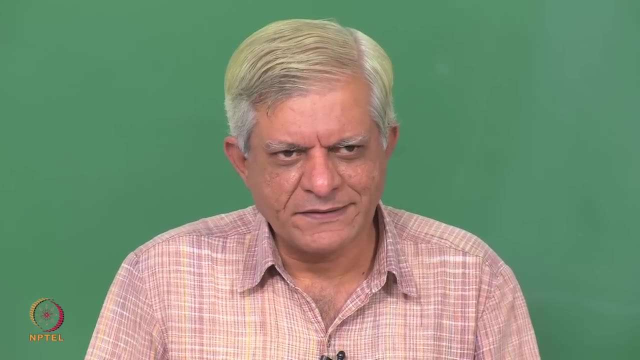 benefit that I am using the word count. or if I say total marks is equal to quiz marks plus quiz 2 marks plus n sem marks, It is only for my benefit that the word marks has no meaning here. So this is not what we mean by meaning. So we will try to define meaning. 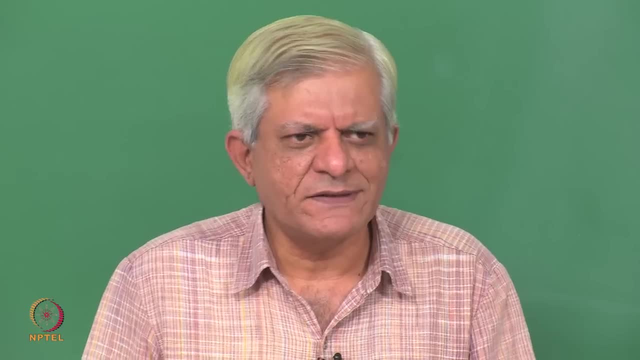 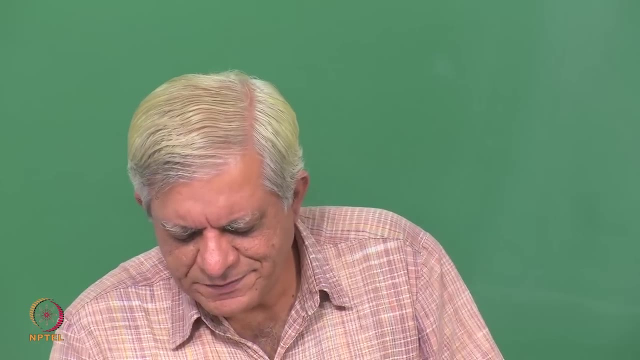 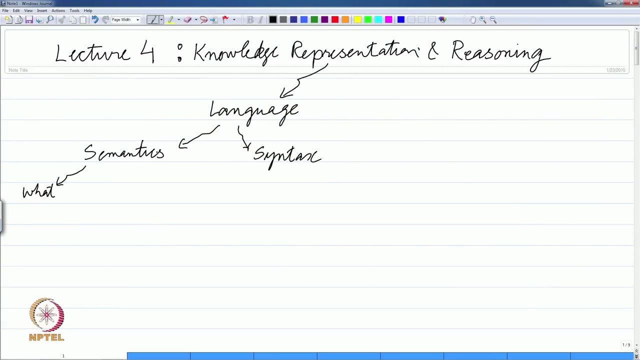 a little bit more formally when we move on to first order logic Today, we will start with the simplest of all languages, which is propositional logic. So just before that, there are two aspects to semantics. One is: what do we mean by whatever we are expressing? 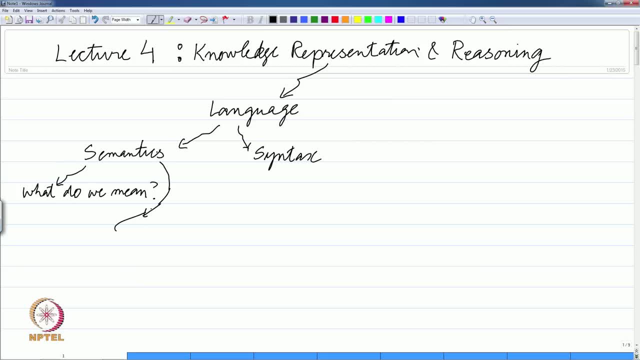 and the second is what you can call as truth functional semantics. By this we are concerned with the truth, value of statement, essentially. So we said that we are looking at classical logic or two elements: True valued logic. So in our case, every sentence will be mapped either to a value. 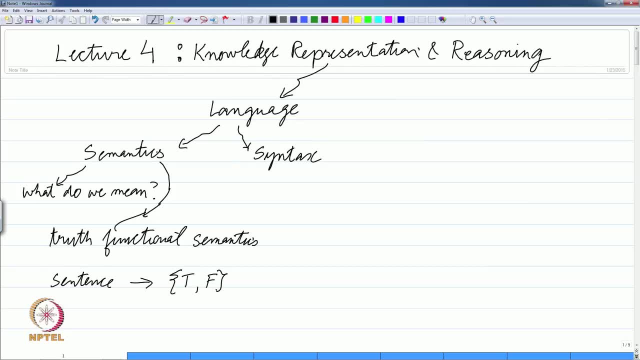 true or a value false, So which we could also write as true or false, or we could write as 1 comma 0.. But basically it is a two valued set, One of them which we interpret to stand for sentences being true and the other we intend to stand for sentences being false. essentially Now, 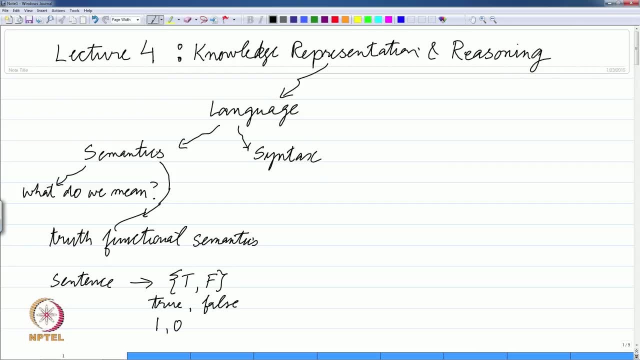 when it comes to syntax of the language, we essentially need an alphabet, And from this alphabet we construct a set of formulas or sentences. We often use the term well-formed formulas, So it is. it is kind of conventional to use the word formulas as a plural, though the 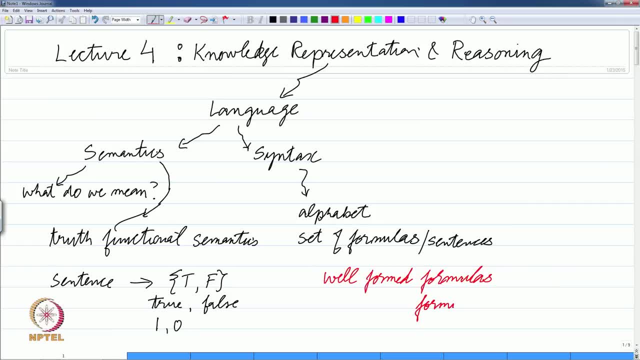 older style used to be: you would say formulae. it does not matter, we will use the term formulas, you can see. So this is what we mean by the term formulas. So when we say formulas, we mean a well-formed formula. it basically means that a word in 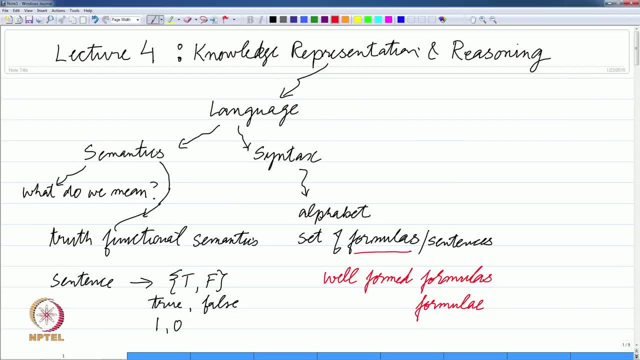 the language that you are trying to define. you can see, When it comes to reasoning, we will basically mean inference. you can see, which we can interpret as saying: what else do we know, So, what else do we know So we? 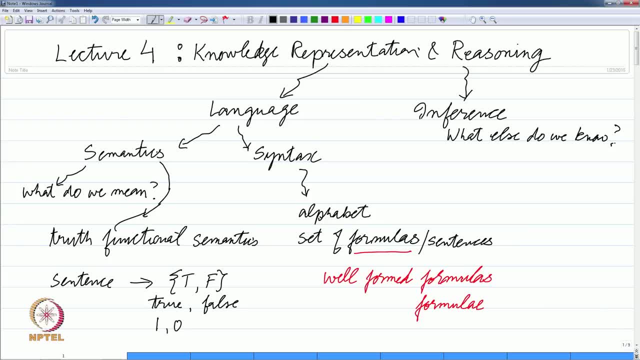 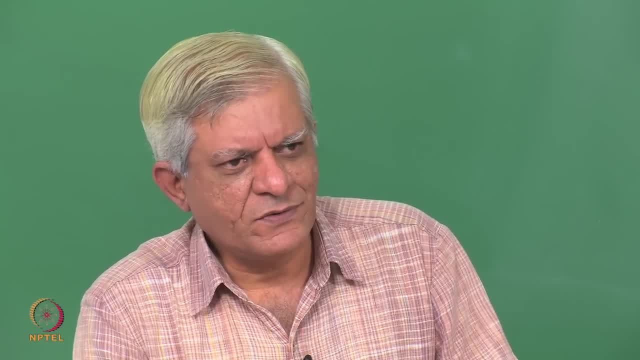 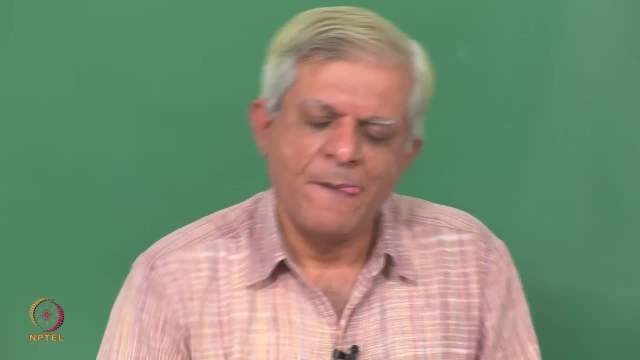 answer it as say: you know, you know something from your own abilities, So you know it from your examples of actual chests. so also that is the basic there. So essentially the basic idea behind this whole effort is that, given that you know some, 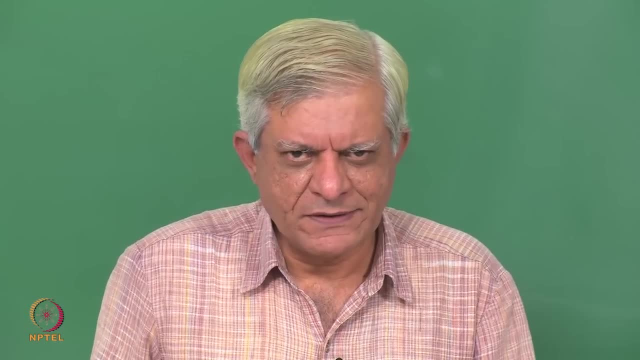 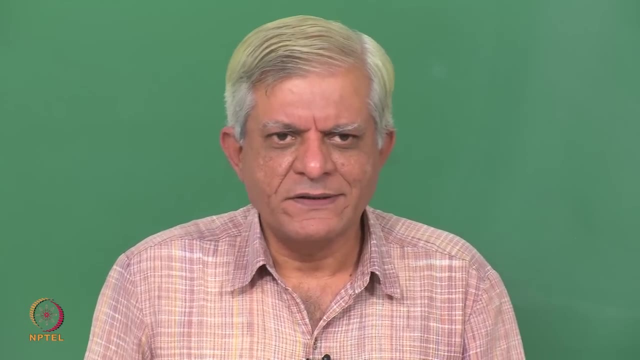 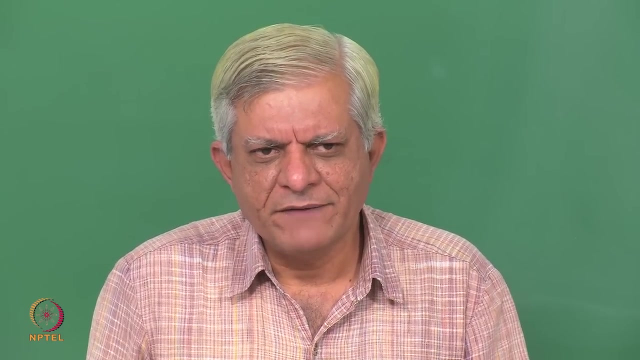 things. you know some facts. So essentially that, what else can you say that? And if we know that Socrates is a man, then we also know, even though it is not stated, that Socrates is mortal. essentially So, that is the kind of reasoning we want to do. 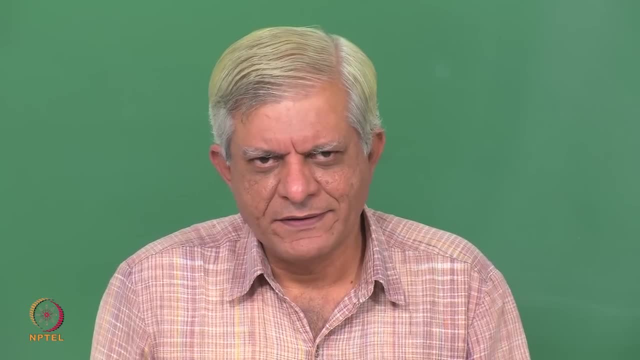 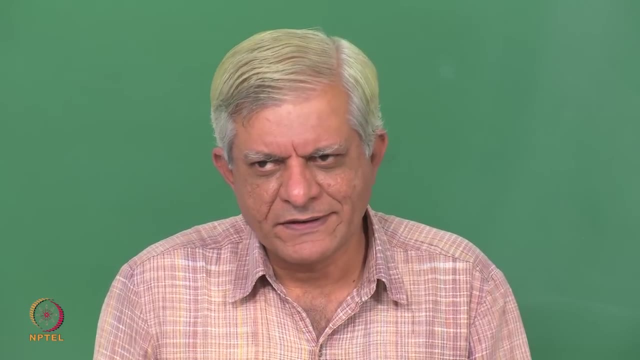 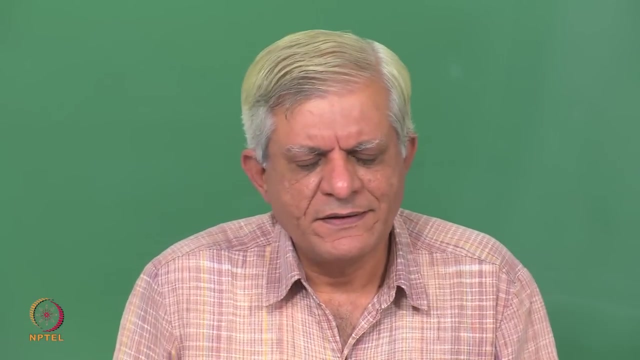 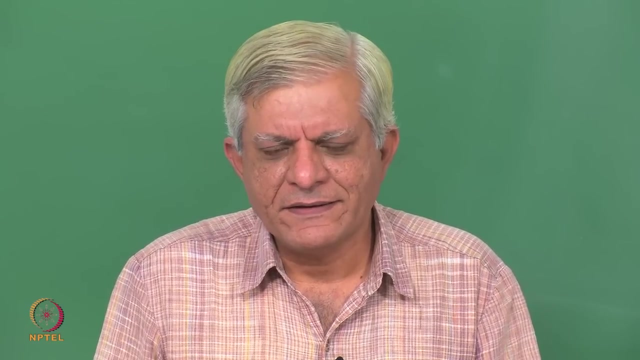 And we will see that reasoning can be of different kinds. In some places you are sure that what you infer is true. in other places it may not be true. essentially, We also mentioned that there is a whole family of languages which logicians have defined, and they differ. 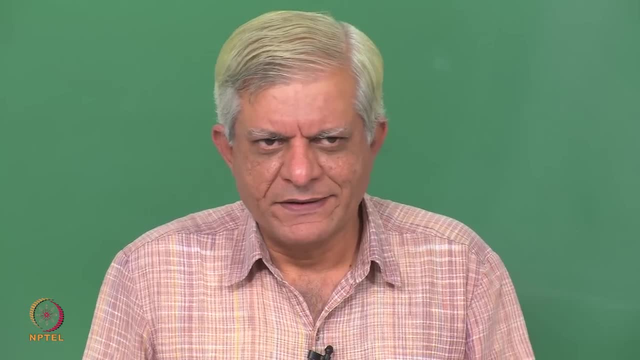 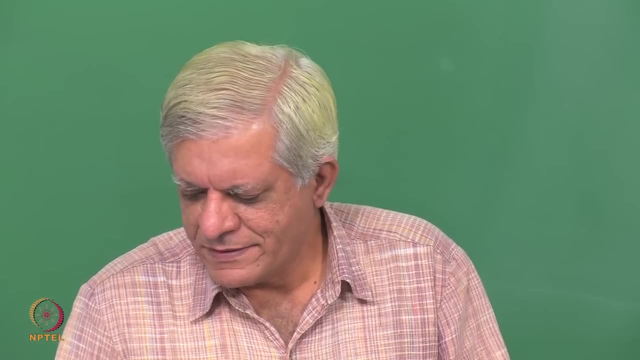 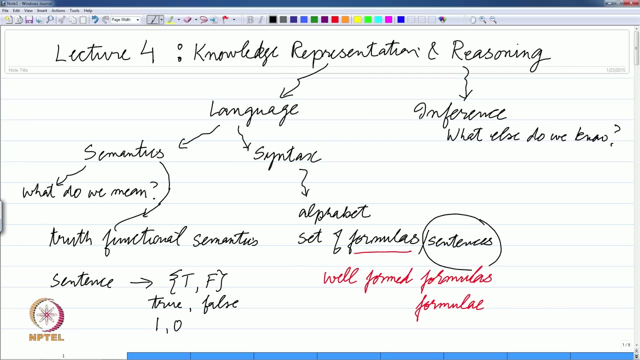 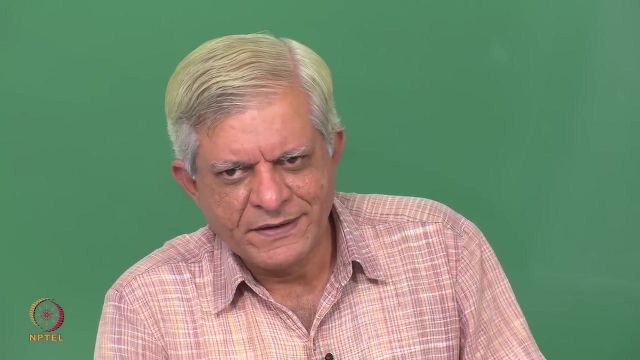 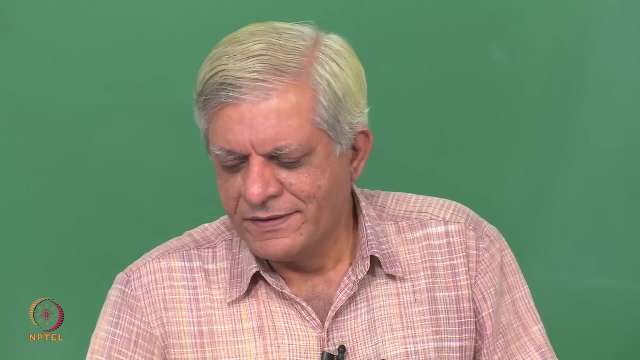 in how much do they allow you to express in a sentence? But the basic unit of logic is something called a sentence essentially. So a knowledge base essentially is a collection of sentences. And again, you can, you know whatever federal regime action, you can also say whether the 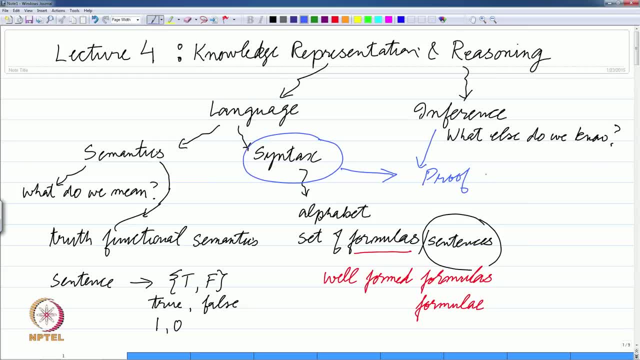 religious sees it as a religious feeling or the moral. So the word society has given to it is this: big, that is a political system, but general terms of social culture are not those of system. So this can be from Europe, as you can say. obviously. 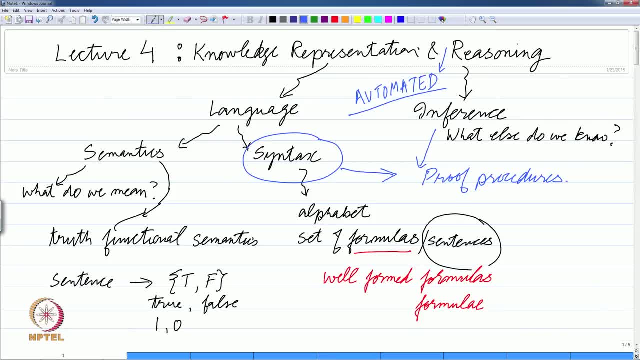 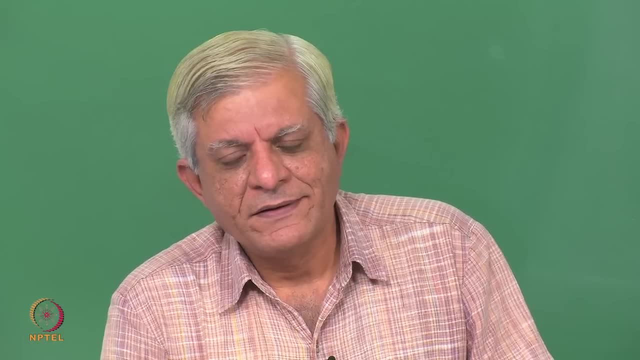 Since we want computer programs to do the reasoning for us, we will be interested in those approaches or those algorithms which can be implemented over this logic system. So at the beginning- may be today, sometime- I will show you that there are proof methods. 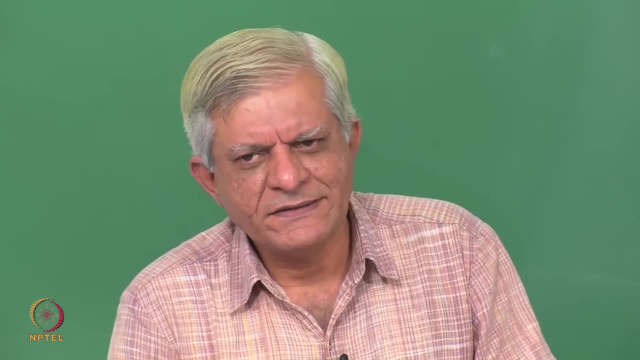 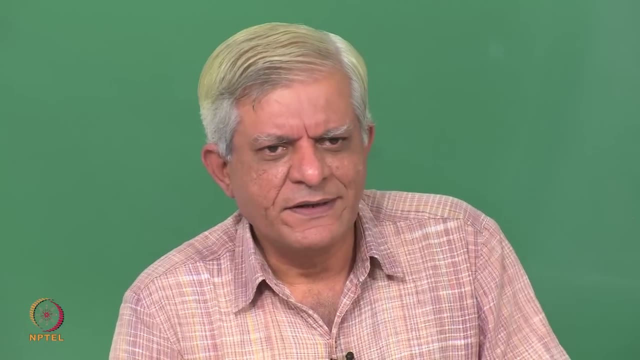 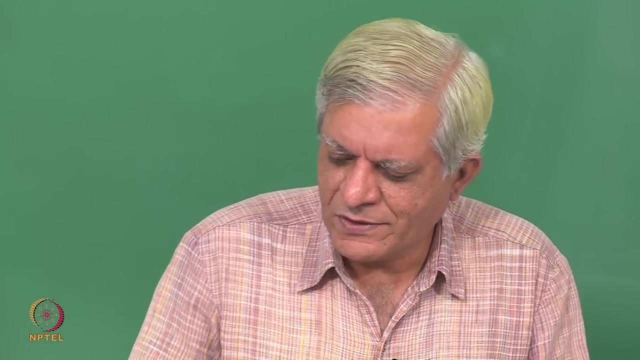 which are difficult to implement in algorithms, essentially because they essentially involve making guesses or making choices, which is easy somehow for us to do at this moment, but it is not easy to put down in an algorithm. So as we go along this course, we will sort of oscillate between representation and 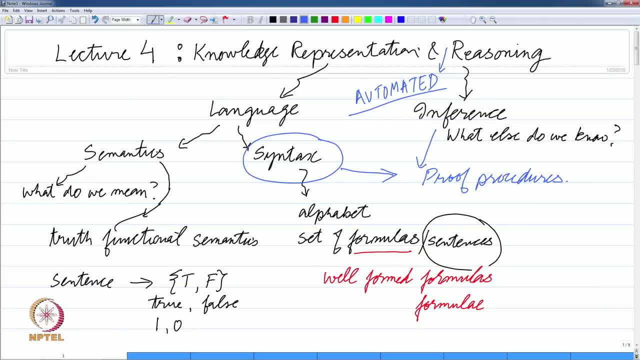 reasoning. Representation is our concern as to how can we represent what we really want, what we mean or what we want to say essentially, how expressive the language is, how can we represent complex facts essentially, whereas reasoning is concerned with the proof procedures and the algorithms that we will apply on the representation essentially. 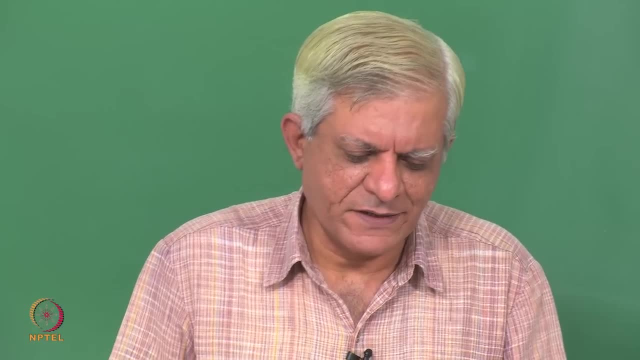 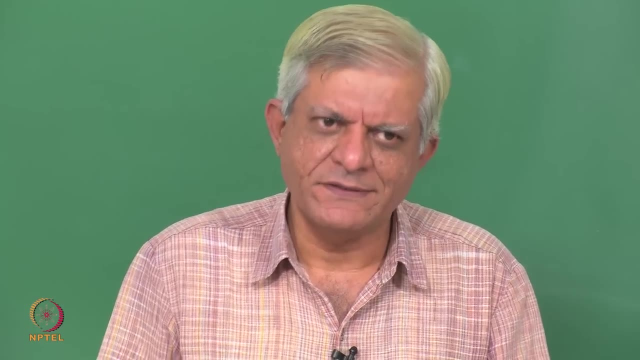 So when you look at the kind of domain of logic, then there is a whole class of people who are you might call as theoreticians or mathematicians or logicians, who are not so much concerned with representation. So they will assume that you somehow they will tell. 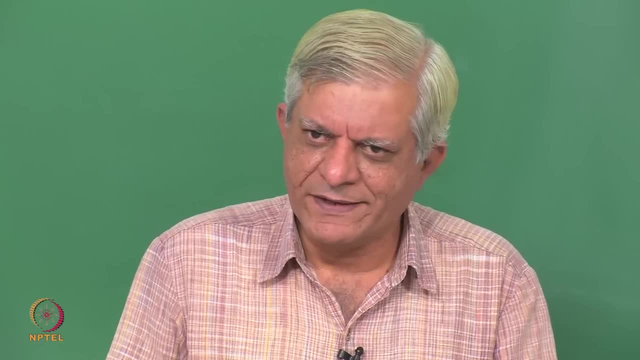 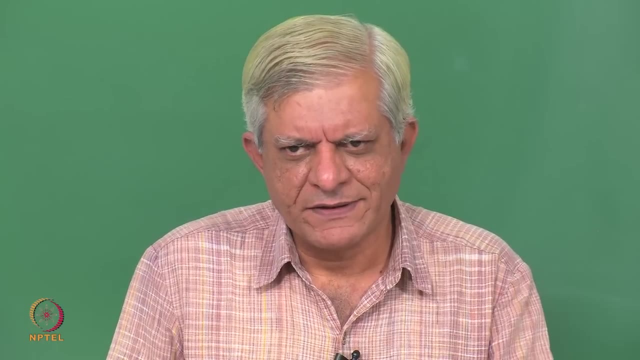 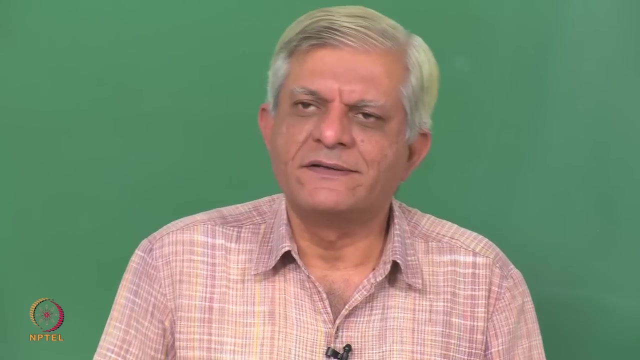 you, this is the language and somehow you represent what you want to say in that language, but they are more concerned with reasoning and things like you know whether the algorithms will terminate and whether everything can be inferred, and completeness that we mentioned last time, Whereas as somebody who may be wanting to develop applications, you would 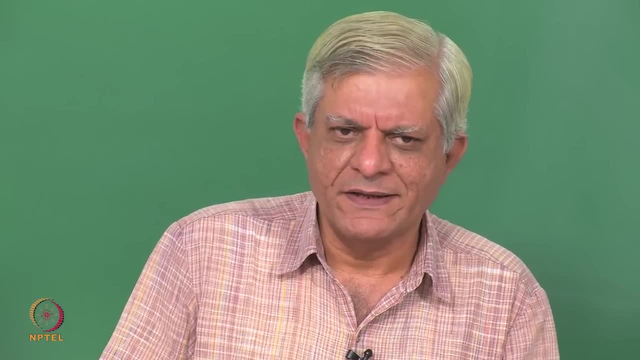 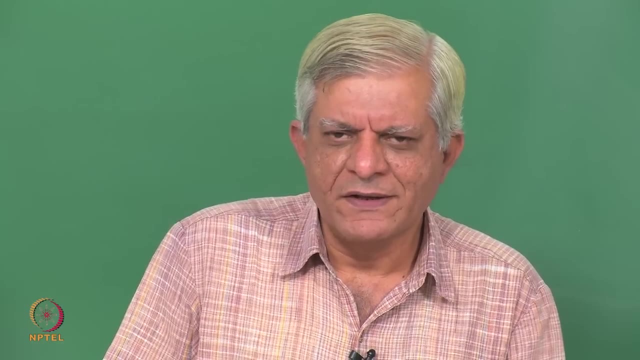 also be interested in representation. So how can you represent what you want to represent? and we will see that that is quite a involved subject. essentially, It is not so straightforward to represent all kinds of things that we can express in English. English, as we mentioned. 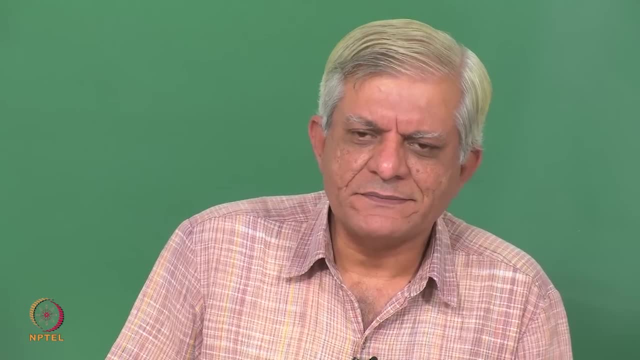 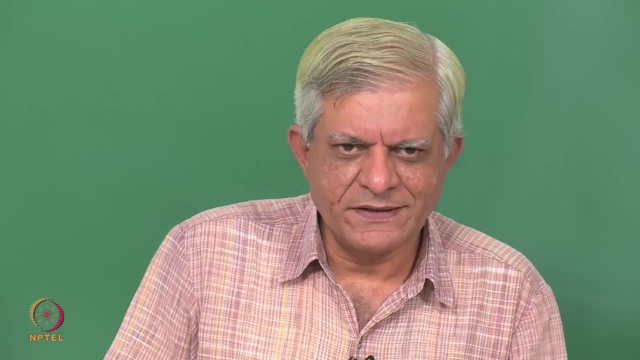 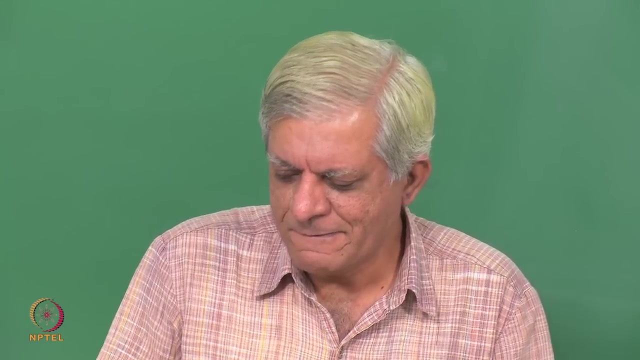 is all Hindi, or Tamil for that matter- very expressive languages. you can say a lot in that, but also it is difficult to interpret or difficult to parse essentially. So you must have encountered situations where you have ambiguous sentences. it is not so easy to parse essentially. 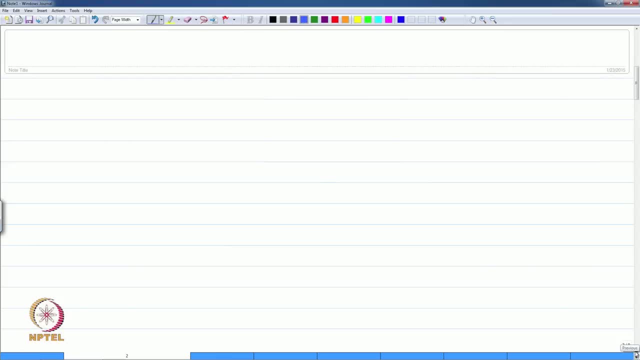 So let us just look at what we meant by reasoning at a very high level. So what we have is that a knowledge base- So we will use the term KB, for a knowledge base- is set of sentences. So when you say a set of sentences, we also mean in some language. 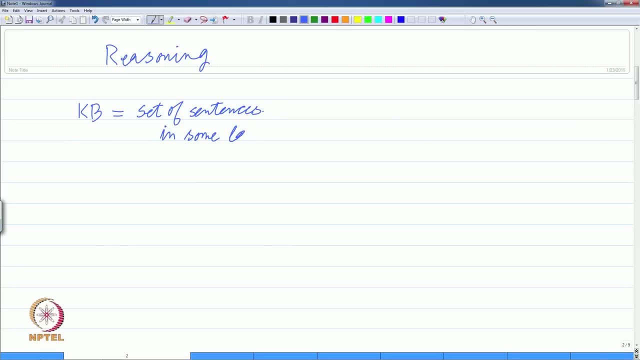 basically saying that there is a single agent And, in effect, we are basically reasoning. 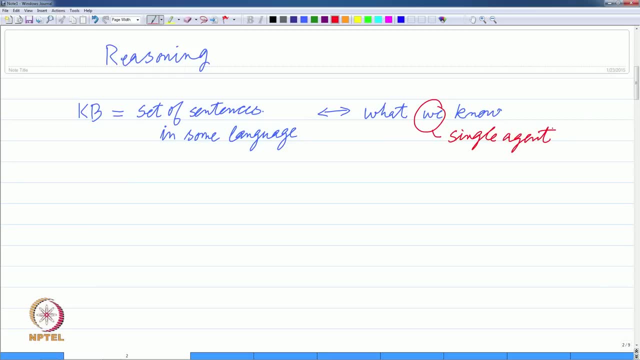 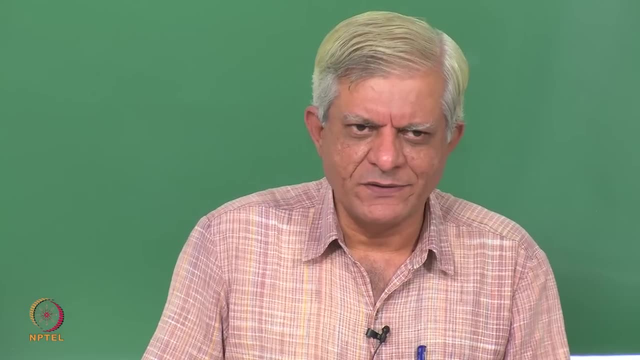 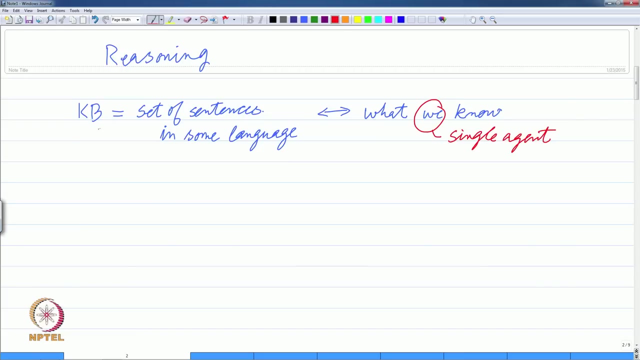 on behalf of that single agent. So whenever we say that there is certain sentences in a knowledge base, we essentially are saying what does that particular agent know essentially Now? so we can kind of represent a knowledge base by a set And it has a set. 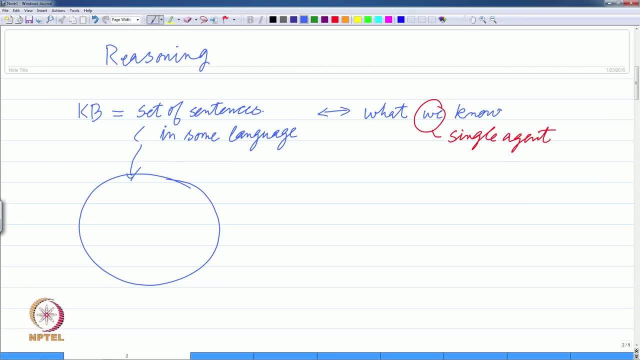 of sentences in that. Now the semantics says that whatever is inside, this is true. So when you say that you have a set of sentences, then you are assuming that what is given to you is true. So if you have the sentences, 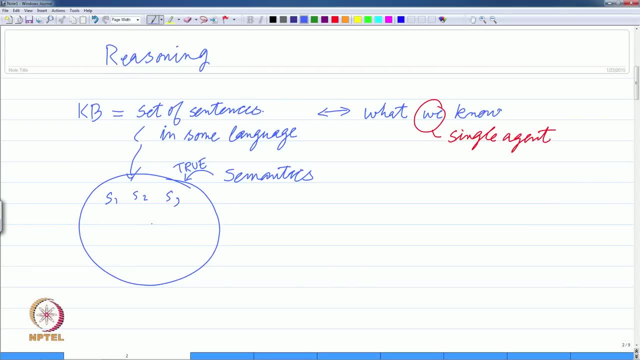 S 1,, S 2,, S 3 and so on. then essentially, you are saying that what else is true? Then, in reasoning, what you are asking is: what else is true? That is what we said. What else do we know? 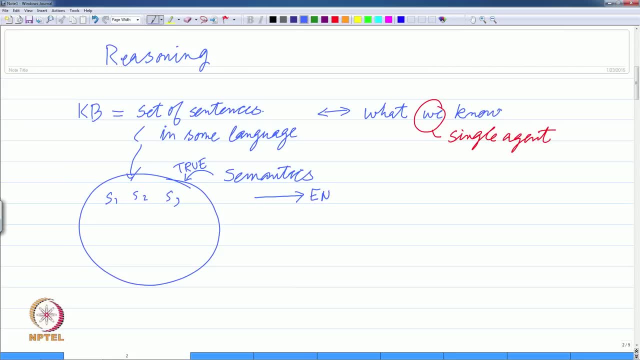 The term that we use is entailment And we want to ask in general whether a given such is true And what else is true. that is what we said. What else do we know? sentence alpha. So, given a set of sentences which we assume to be true, entailment defines: 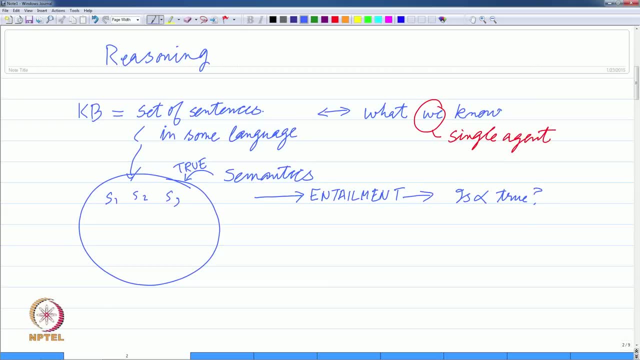 the set of sentences which are also true as a consequence essentially, which are necessarily true as a consequence. So that is what we had said. That is the notion of entailment, essentially, Whereas reasoning is concerned with a proof procedure and the question we ask. 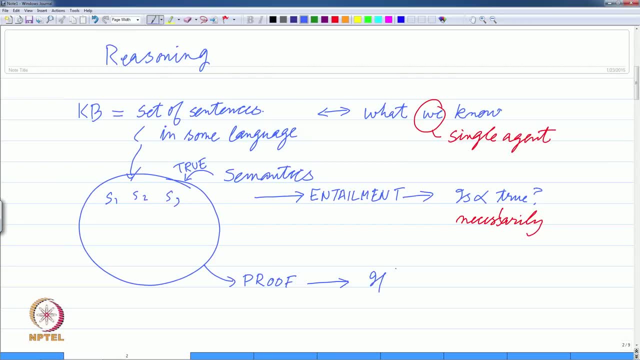 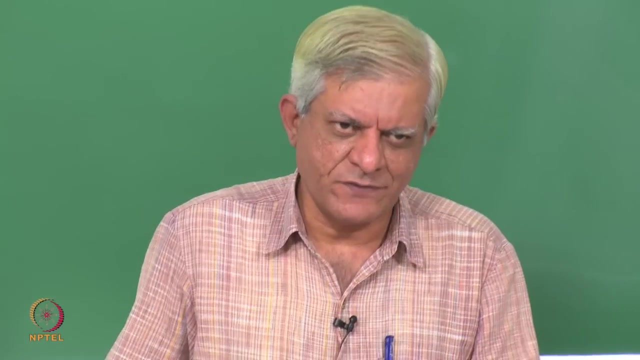 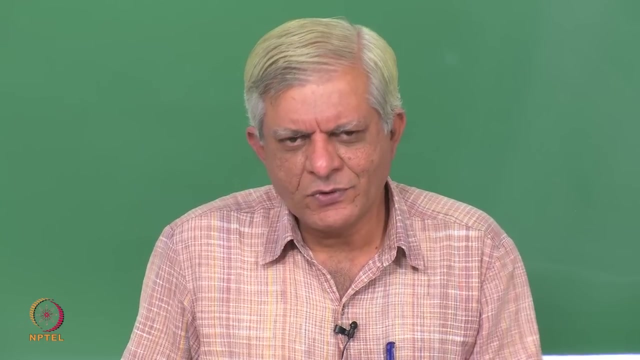 is So. the proof procedure is alpha, alpha, provable. and when you say provable, we will say: by our 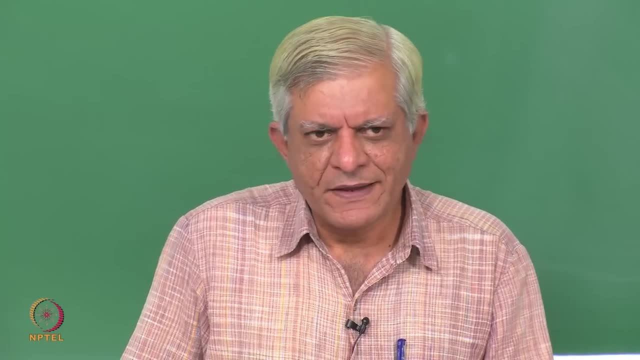 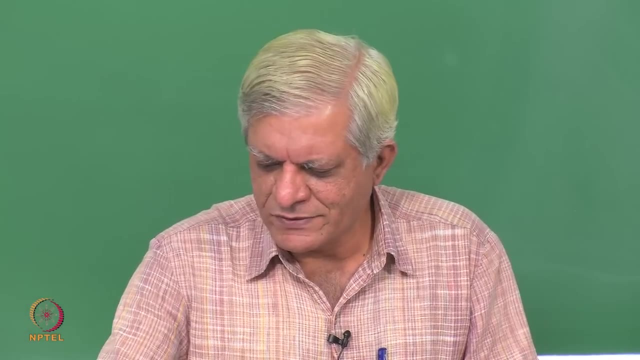 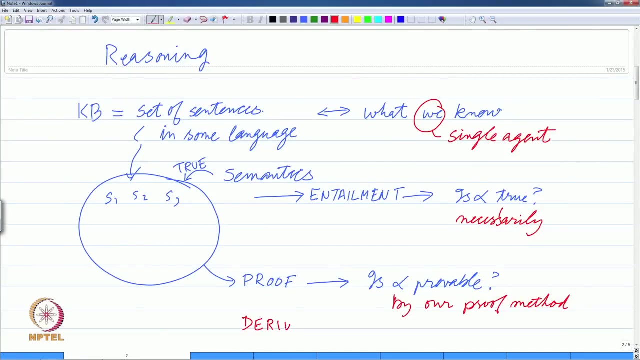 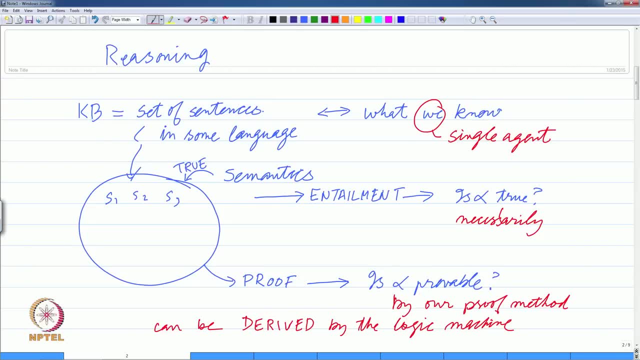 Yeah, so by true you mean something that is necessarily true as a consequence, and we 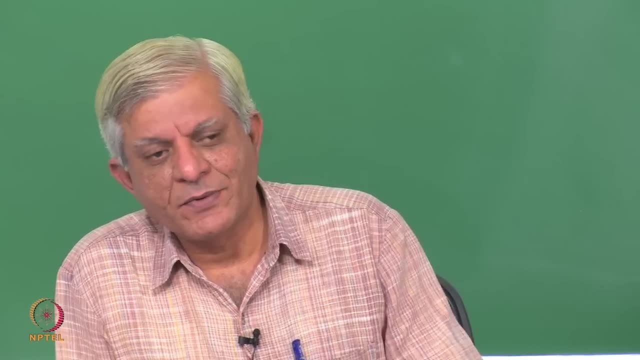 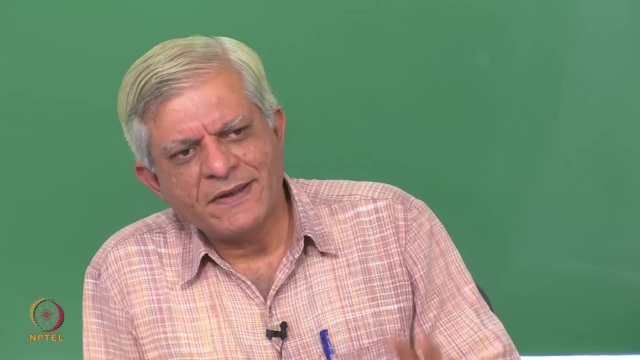 will define this very shortly. when we define the proportional language language, we will see what do these mean in that context. this- I am talking at a very general level, but true- is a semantic notion. so if you know fact A, fact B, fact C, fact D, what else is true? as 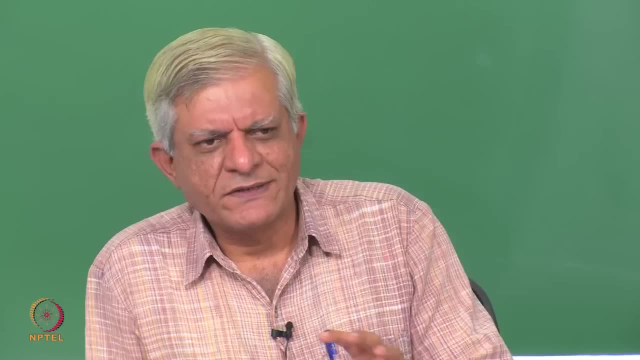 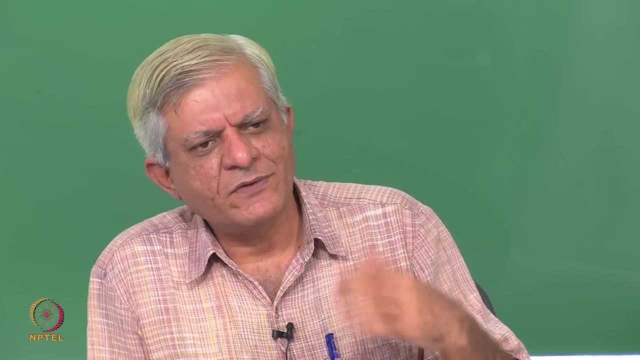 a consequence of that is necessary. that is the notion of truth. it is a semantic notion, Whereas proof is a syntactic notion which says that can you write an algorithm which will take the given facts of the given to you if you have fact A, fact B, fact C and 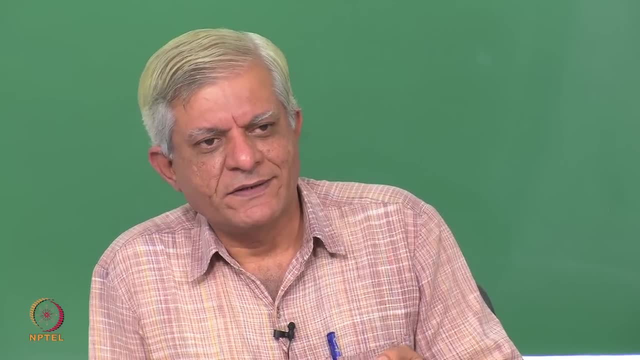 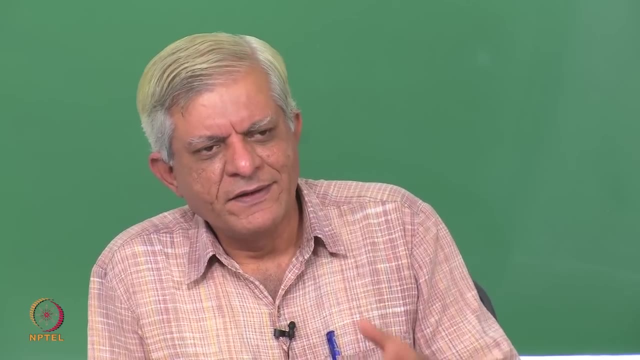 fact D. what else will the program produce essentially? So the program is just. it is just a program which looks at what it has and applies some rules, as we will see, and produces new sentences. So this production of new sentences is a syntactic process and we refer to that as a proof, essentially, And we will 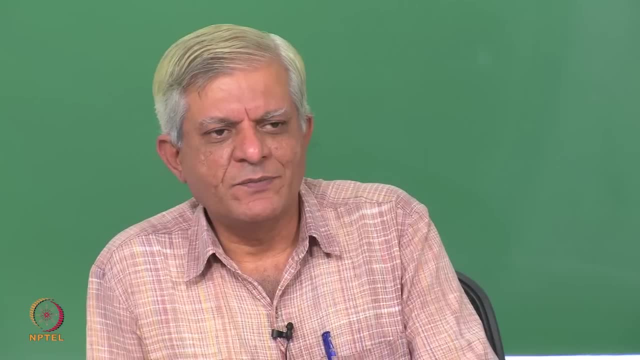 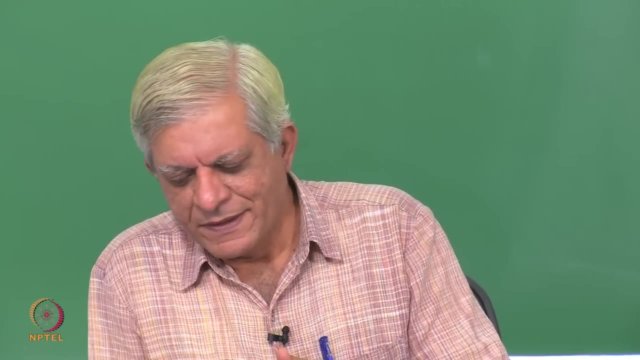 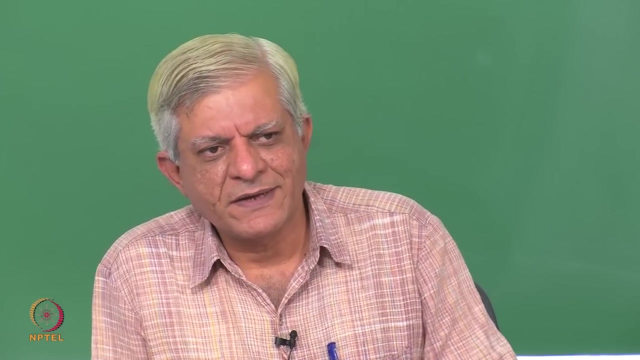 see that, what is the conditions that we will put on proofs? essentially, what constitutes a proof? what makes a proof a proof? we will look at some of these things shortly. essentially So, it is a mechanical process. the process of generating a proof is a mechanical process. 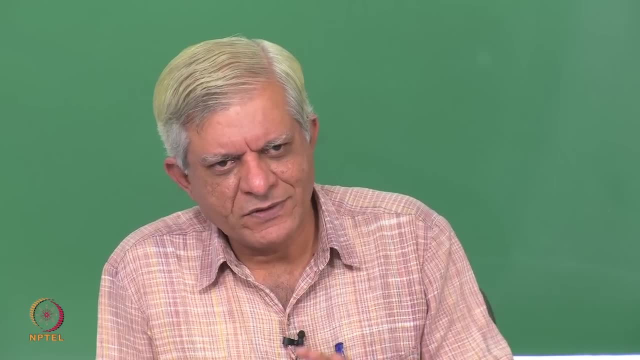 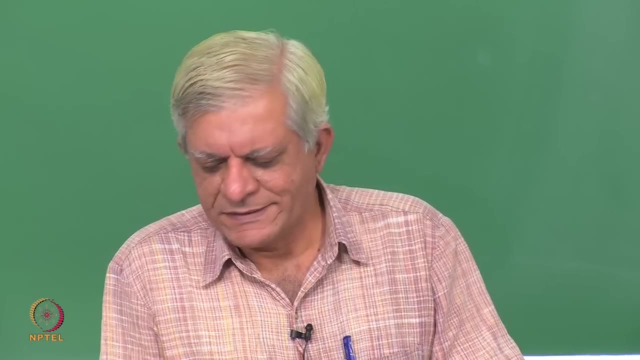 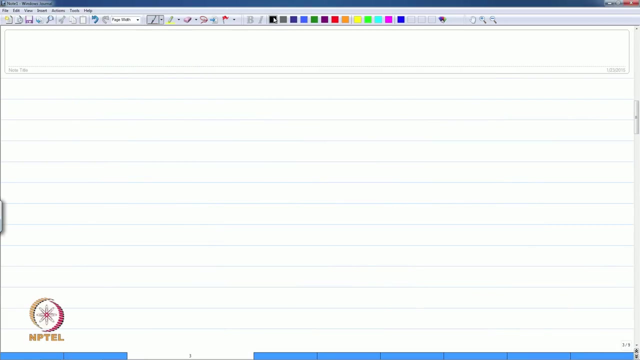 in the sense that you do not look at the meaning of the word, you only look at the form of the relations between words. And as we go along, I think this will become a little bit clearer. So we begin with the simplest of all languages, which is proportional logic. So first we 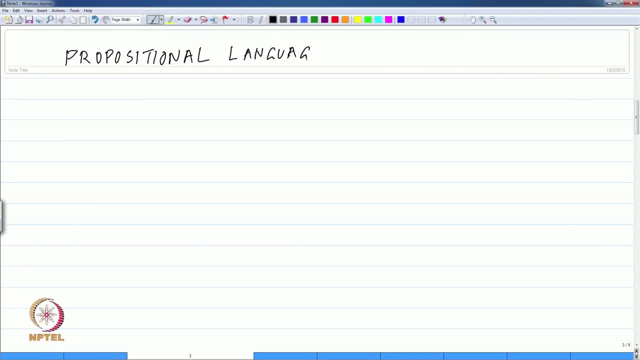 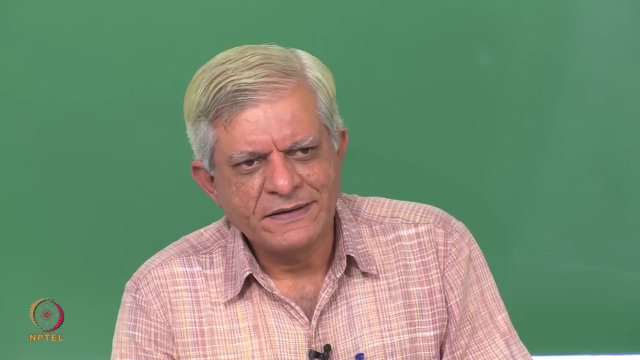 define a language called a proportional language, And the distinguishing feature about proportional language is that sentences are atomic. We cannot break down a sentence any further, we can only treat it as an atomic entity. it is atomic unit which is defined in this language essentially. So any sentence that you want to reason about will be treated as 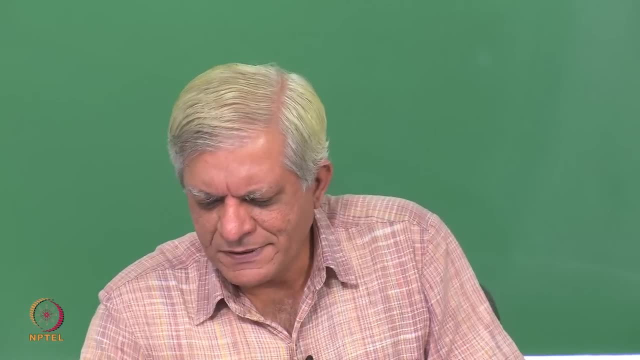 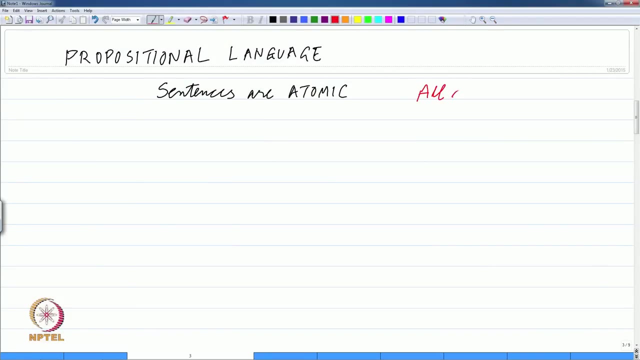 an atomic entity example. if I want to talk about the sentence all men are mortal, then in proportional logic, I will simply say that this corresponds to a sentence which I will call p. So we will be working, as we will see shortly, with proportional. 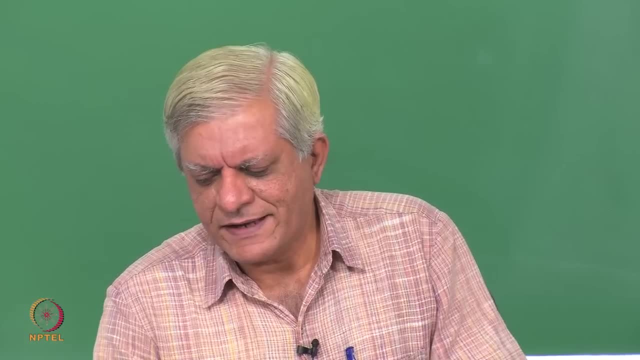 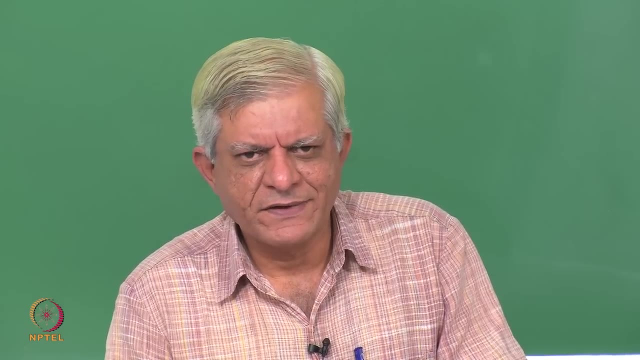 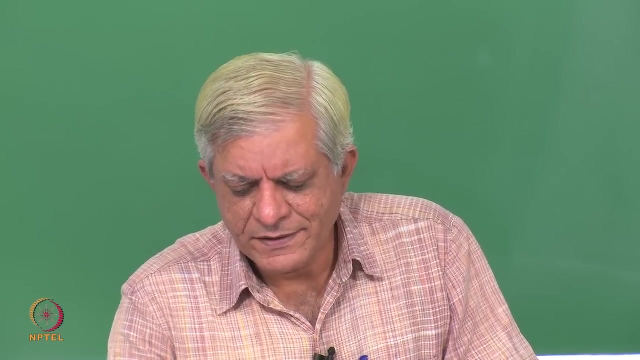 symbols or proportional variables which will stand for sentences. It is up to us what we want to plug in into p, but as far as proportional language is concerned, one sentence is denoted by one atomic variable, essentially. On the other hand, when you look at F O, L, 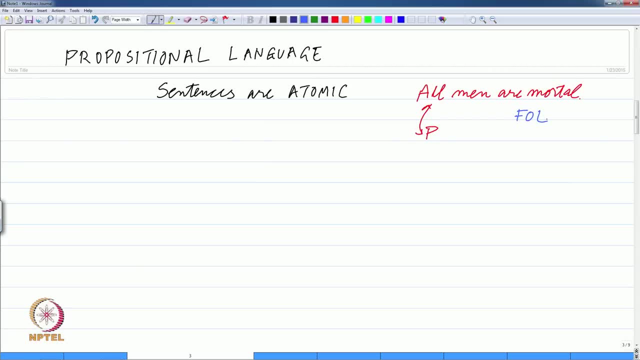 first order logic, which we will do in due course of time. we would represent this sentence by breaking it up into smaller parts. We will write it something like this: If you do not know this language, it does not matter. For the moment, you can simply say that we 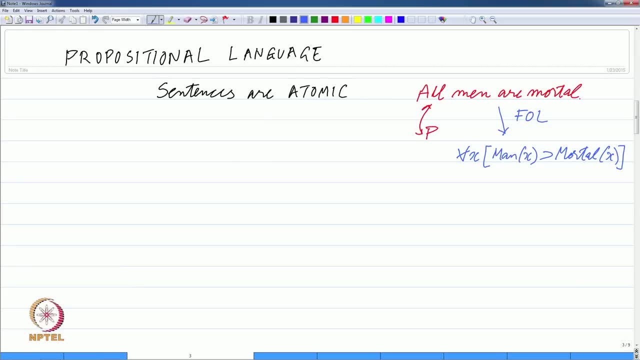 are distinguished between categories of things called men or humans and categories of things which are mortal. And all we are saying is in this expression is that for all x. so this symbol stands for all x. If x is a man, then x is mortal. So we are stating the same. 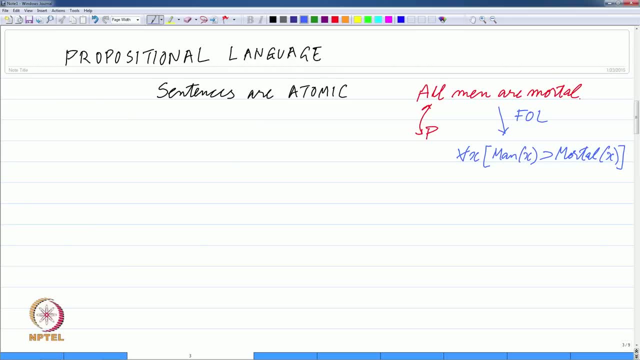 sentence in first order logic, but we have broken it down into parts And you can see, once you break down things into parts, we can reason with the different parts And, in fact, that is what will allow us to eventually relate it to the fact that, because 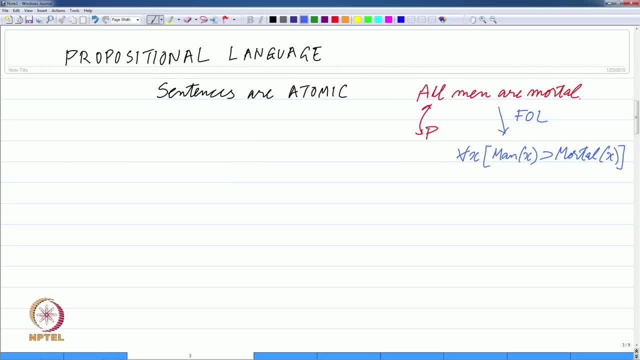 Socrates is also a man, then therefore Socrates must be mortal. But in propositional logic we find that that is, that will not be possible. So this is a key feature about propositional logic: We can think of these as propositional variables. 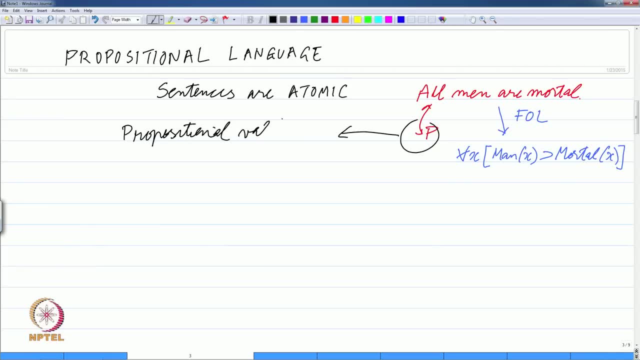 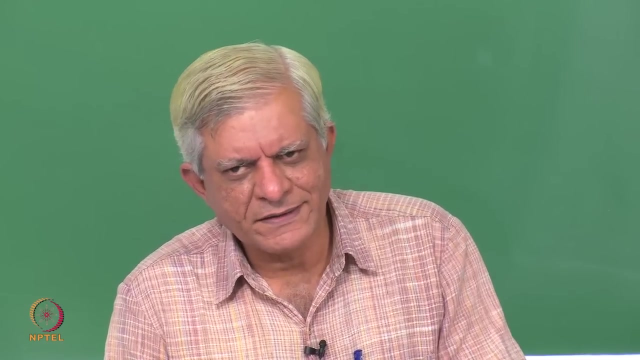 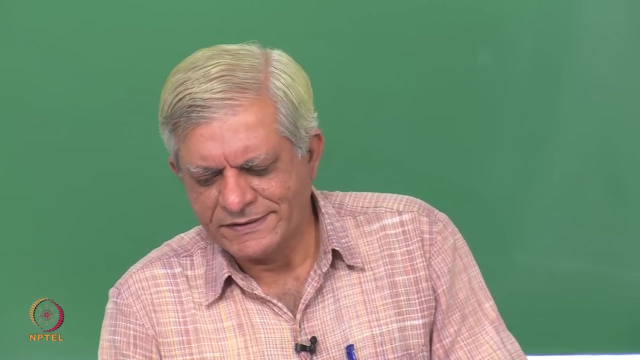 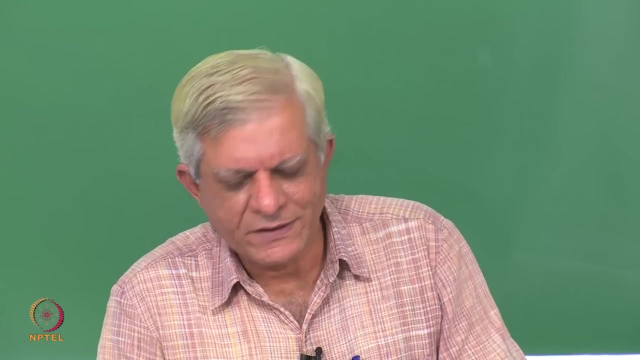 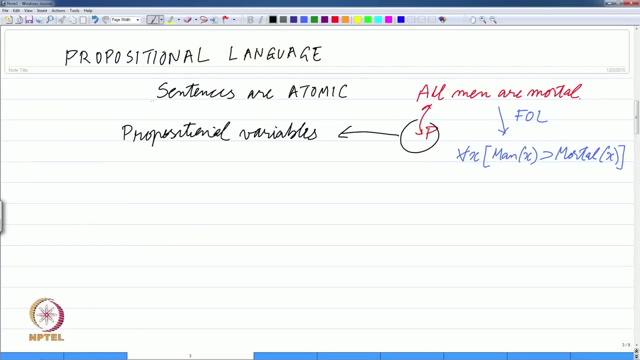 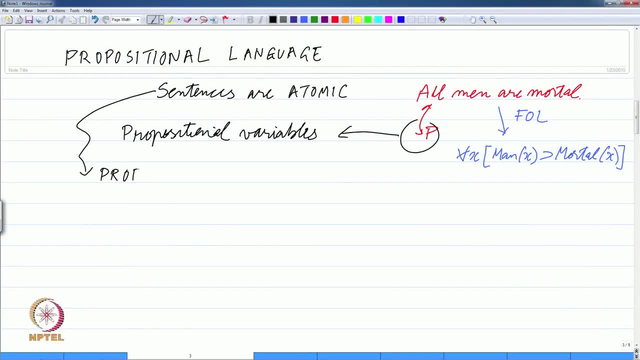 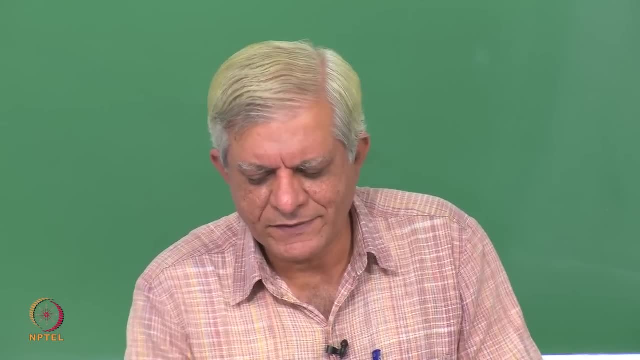 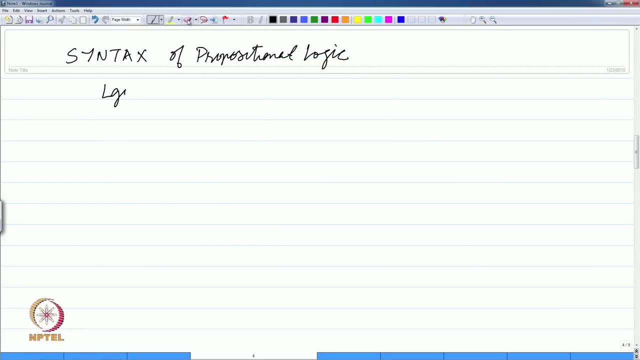 distinguish every language by two parts. one is logical part, and by logical part we mean something which belongs to every logic, every proportional logic. in this case, we are talking about the alphabet. at this moment, every language has an alphabet. the alphabet has two parts. one is a logical part which consists, in the case of proportional logic with things. 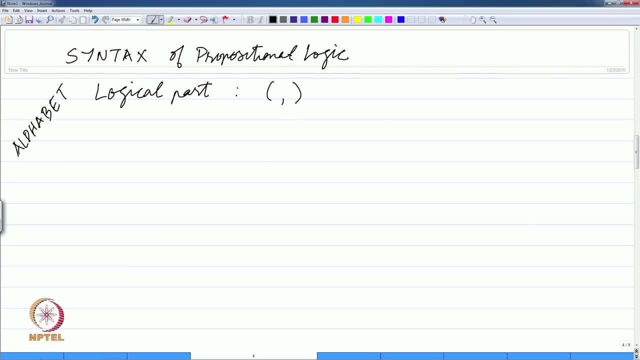 like brackets. So two brackets are in principle enough, but you could also add square brackets or curly brackets To improve readability for us, essentially because we often tend to get confused with many brackets of the same type. essentially, Then we have two special symbols, which are: 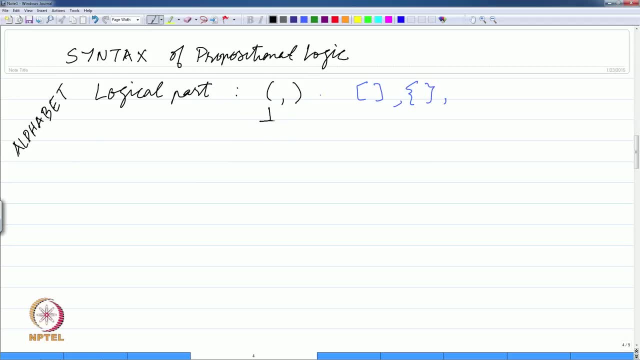 which I will use this notation. These are proportional constants as opposed to variables, but you can use any two symbols essentially. So other people, for example, might use T, f or 1: 0- it does not matter actually- but essentially two symbols. 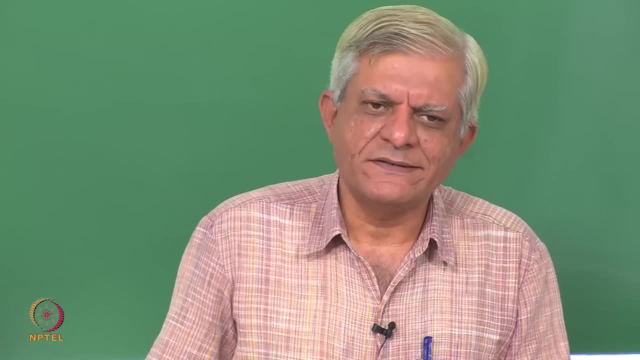 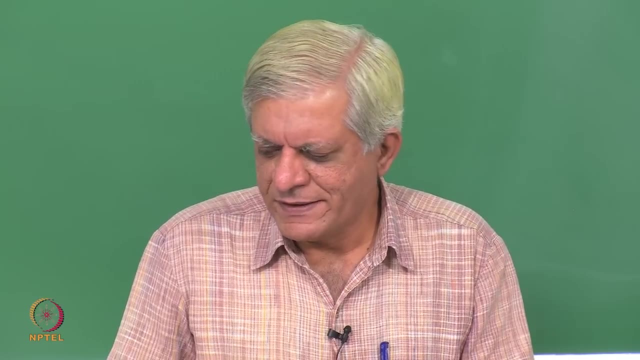 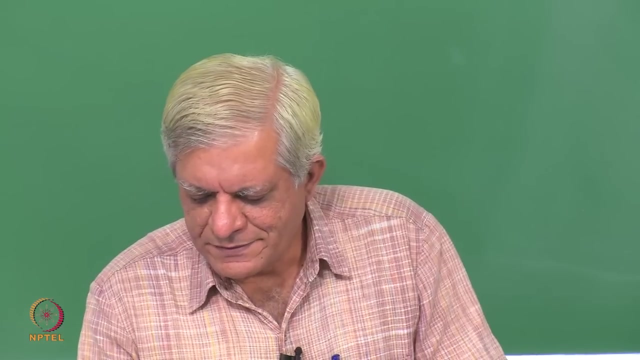 1 will stand for truth. 1 is a stands for a sentence which is always true. 1 stands for a sentence which is always false essentially, and we will represent these 2 sentences by this, So they will be mapped to this 2 valued set that we are been talking about essentially. 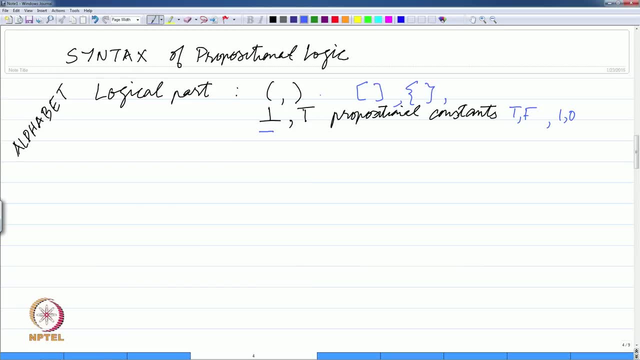 Then we will use a symbol like this. this is a unary connective. sometimes people use this symbol as well. it does not matter, we will use the symbols on the left hand side, and then we have symbols like this. So you are obviously all familiar with this kind of things. 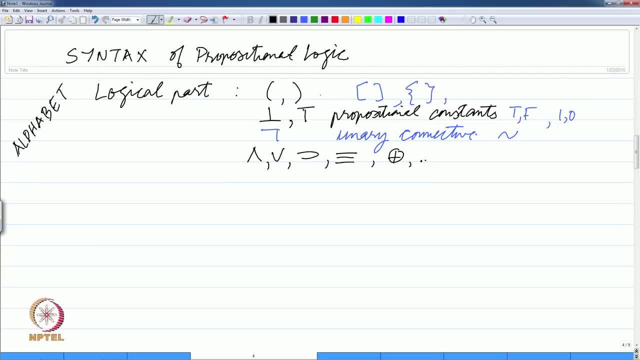 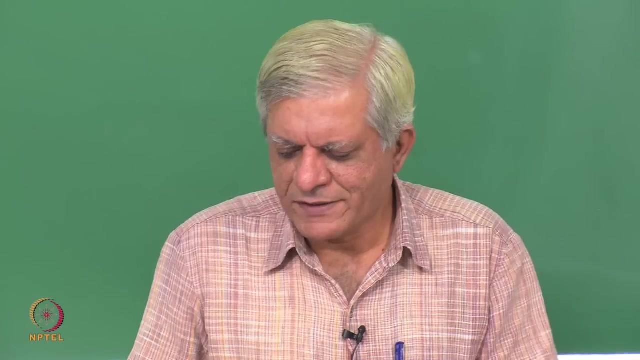 And there are other symbols. some books may use different notations, So instead of this, somebody may use a single arrow, or somebody else may use a double arrow. instead of this, they may use 2 arrows like this, but it does not matter. These are just part of the alphabet. 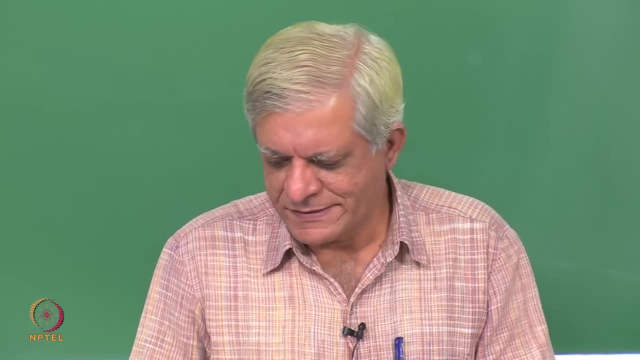 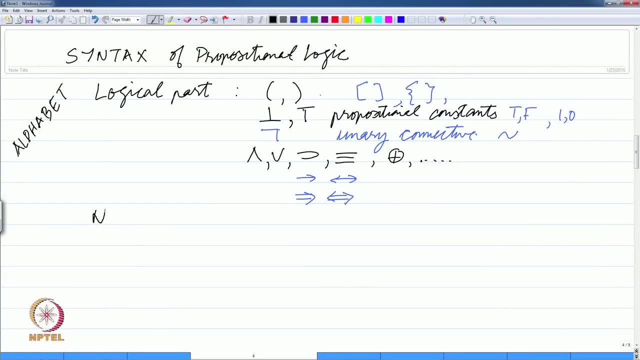 essentially they are used to construct sentences essentially, And the other thing, which some people call as a non logical part, is a set- P, Q, R, a countable set, A set of propositional variables. we also use things like P1, P2, P3 and so on. 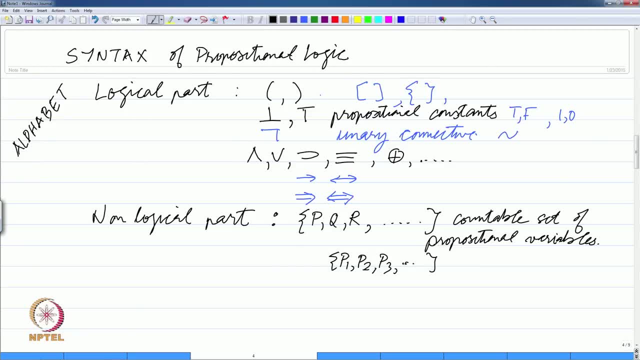 So all this constitutes the alphabet of propositional logic, essentially So at this point may be. I should point out that a given language may choose a subset of connectives. So, for example, you might see somewhere a notation that if you use L to stand for a language, then they would specify what are the